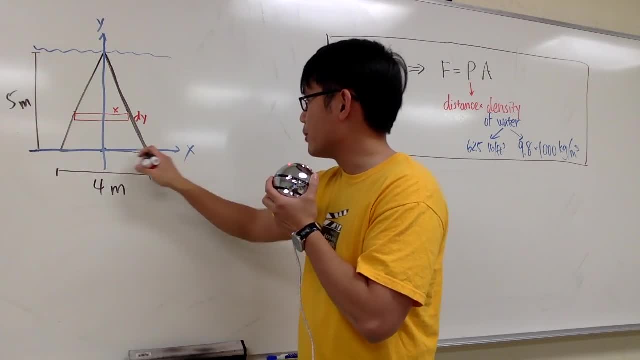 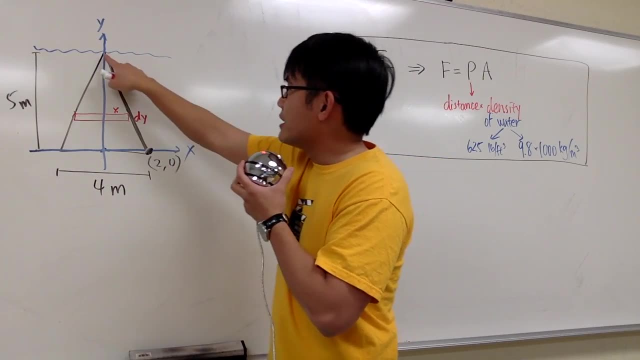 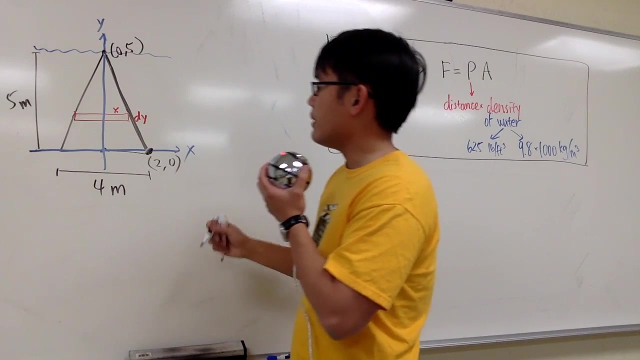 right, But I cut it into half, so this will be 2.. And this is on the x-axis, so this point is 2,0.. How about this point? Well, this is 5 meters, so this right here will be 0,5.. All right, so y well. 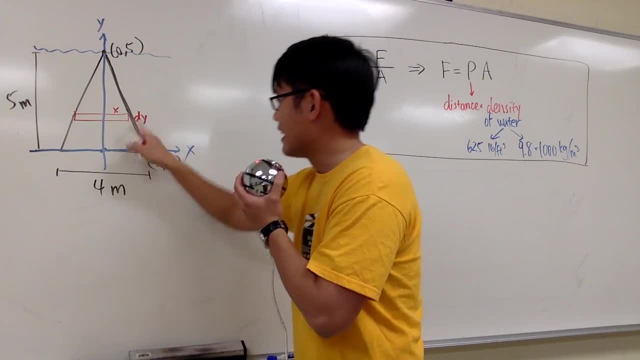 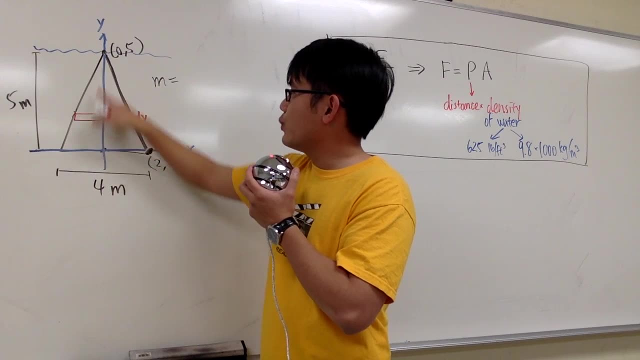 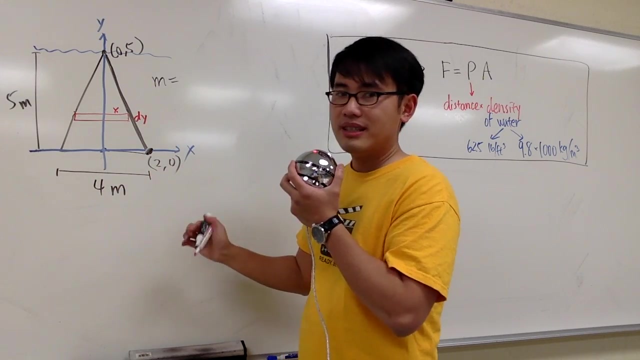 let's get the slope first. What's the slope of this line? This right here will be the y over x right. But then we go down. Look at this right here: We go down 5 units and then move to the right 2 units. so the slope is technically. 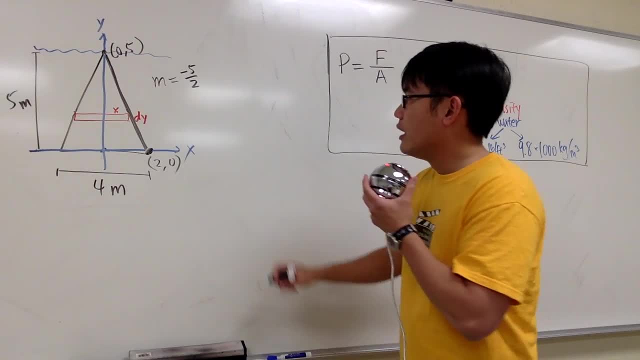 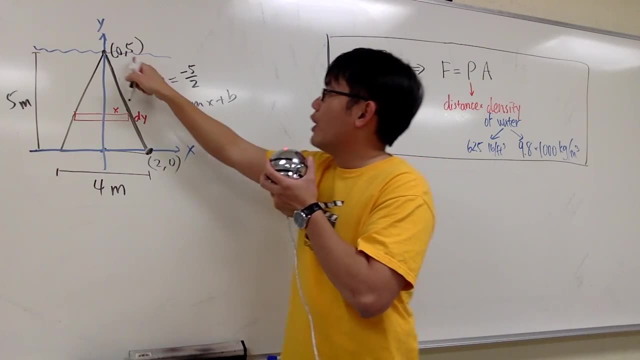 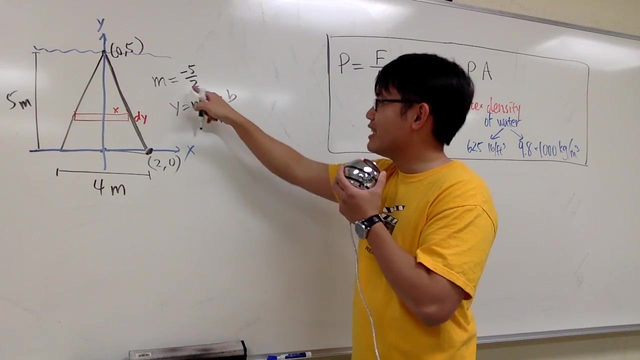 negative 5 over 2.. And in this case we can use: y is equal to mx plus b, And the reason for that is because we know the y intercept right away is 0, 5.. Therefore the b will be 5. And the slope is negative 5 over 2, so this is the. 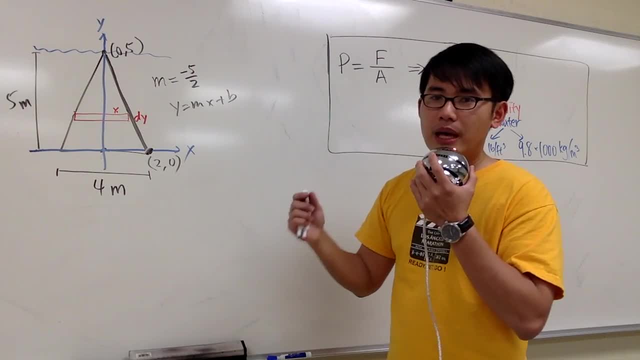 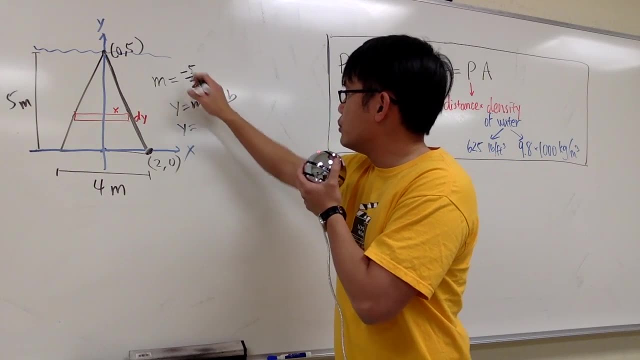 quicker way If you want to use: y minus y1 equals to m times parentheses. x minus x1, that's fine too. Anyways, y will be m, which is negative. 5 over 2x plus b, The b is once. 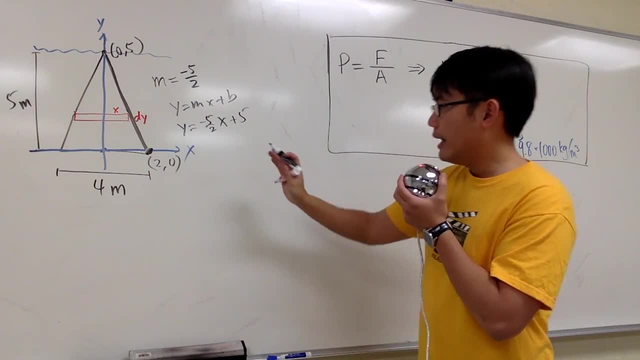 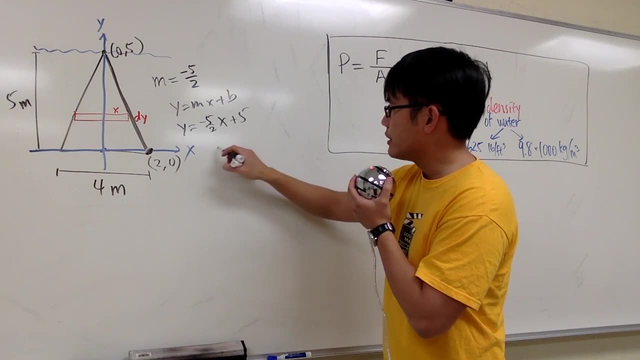 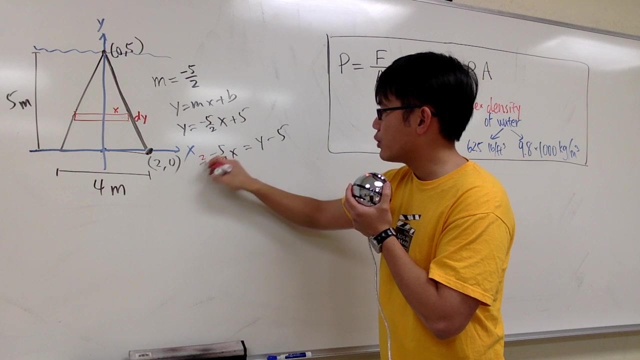 again the y-intercept, which is just the 5.. However, we are going to solve for x. Look at this equation. Let's subtract 5 on both sides, So in another word, we have negative 5 over. 2x equals to y minus 5.. And then I will have to multiply both sides by 2 over. 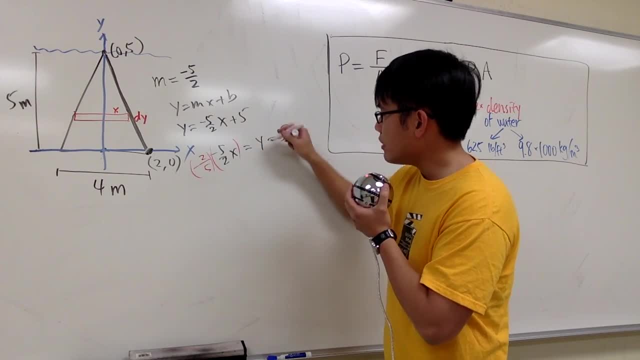 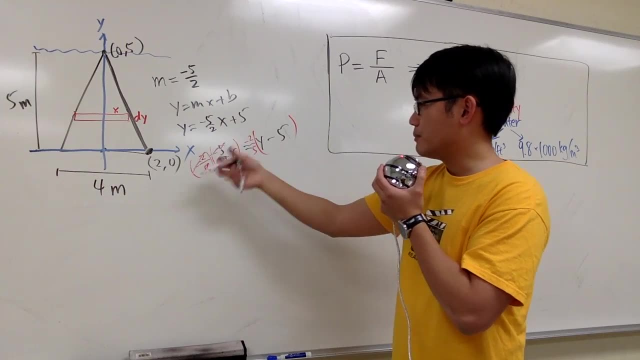 5 by negative on both sides. So squeeze this right here: negative 2 over 5.. So this: with 5, 5,, 2, 2, positive, everything will become positive. on the left-hand side, x will be. 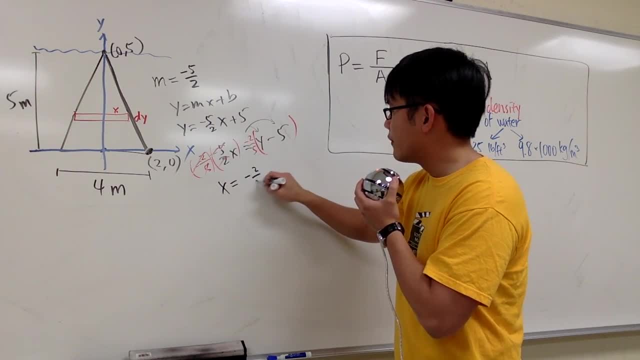 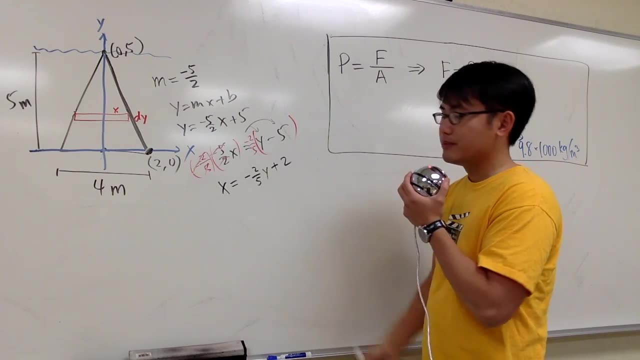 perhaps I can distribute this negative 2 over 5. y and then this times that Negative times negative is positive and then the 5 cancels out. so plus 2. That's x in terms of y, And usually that's the harder part. All right, 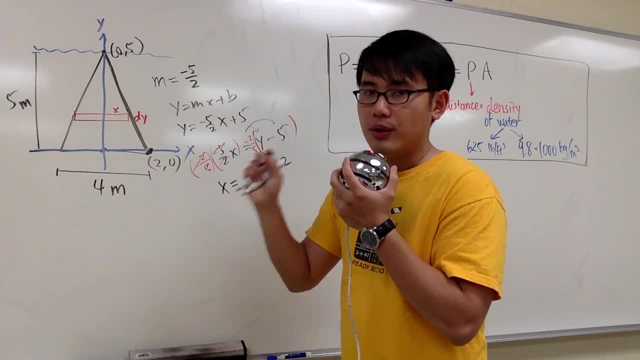 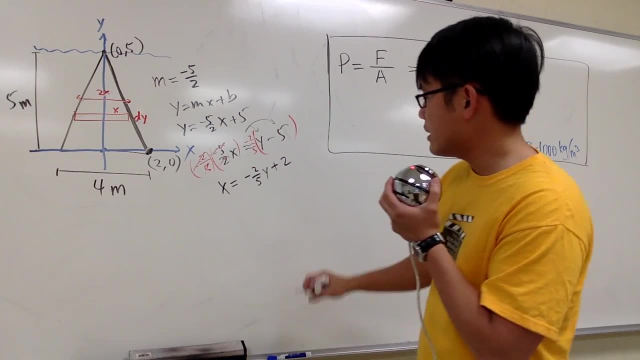 For this rectangle. once again, the area will be 2x, So I'm going to just maybe indicate this right here as 2x. So I would like to put down the integral now. Well, I'm going to put down my integral now. 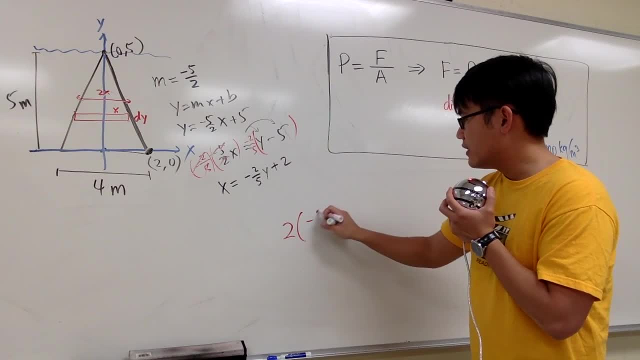 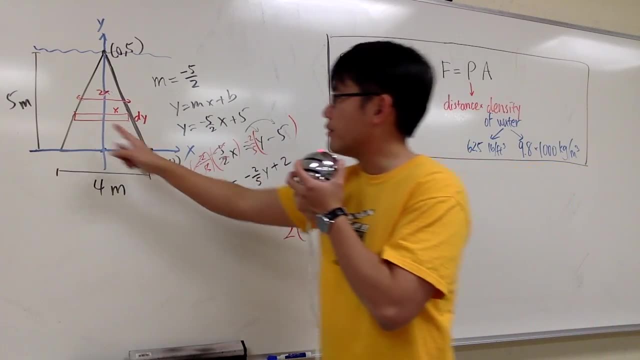 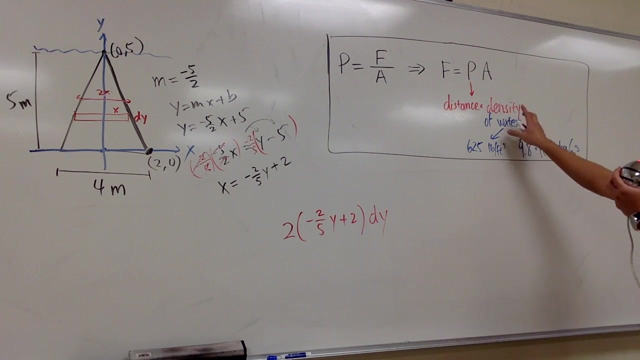 2 times x, which is that negative 2 over 5y plus 2, and then times dy. This right here represents the area of this rectangle. So we are done, The area is, you know, done for that. But then we move to the next thing, which is the density of the water We need. 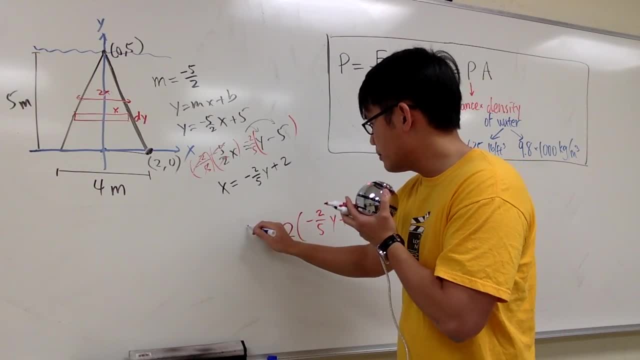 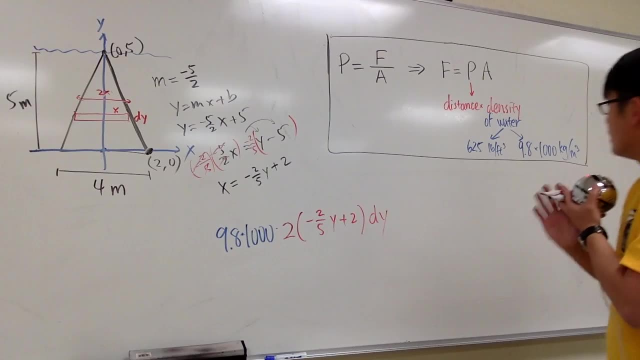 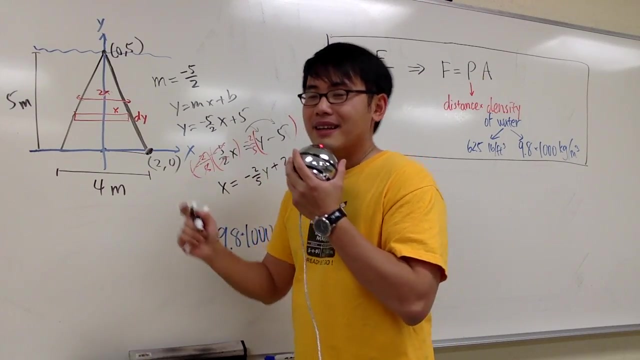 that 9.8 against 1,000.. So I will multiply by 1,000 here and then multiply by 9.8 here. What else do I need? I need the distance now, So it will be based on labeling I have. 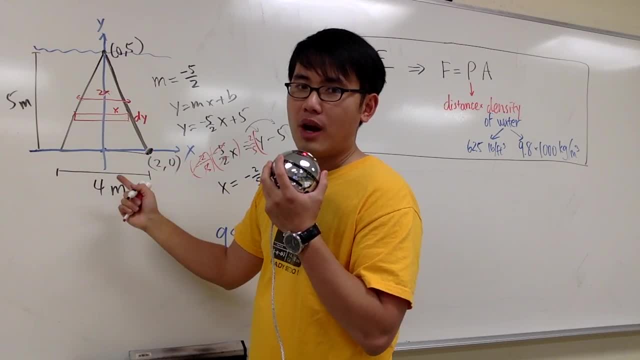 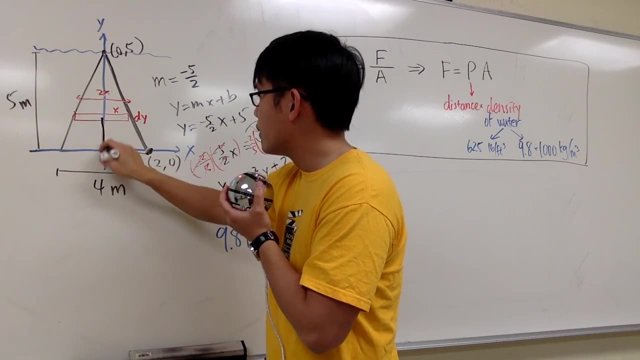 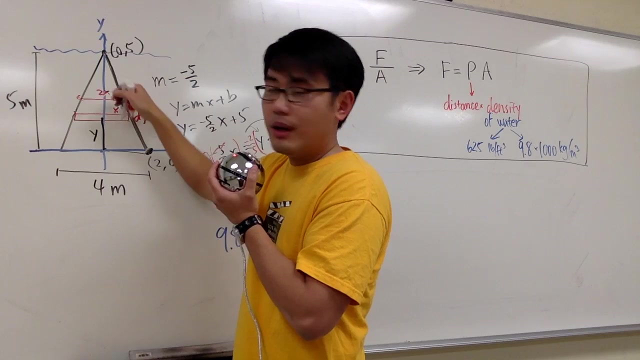 to ask myself how far down is this rectangle underneath the water? based on my labeling, The x-axis was right here. That means from here to here will be the y value. I have to ask myself: what's the distance from here to here? All the way was 5 meters right. 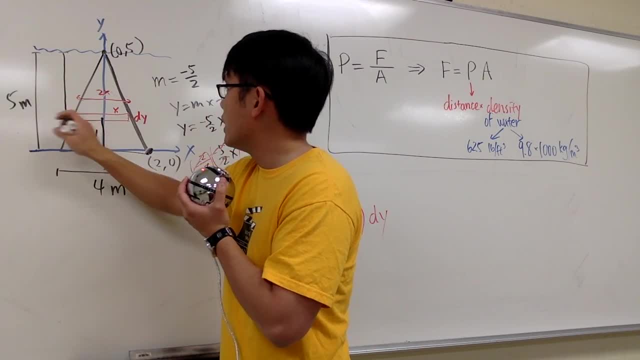 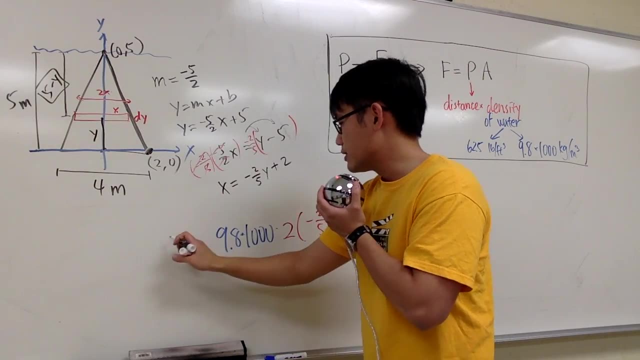 And this much is y already. That means from here to here will be. the whole thing is 5 minus y minus y. So this is the distance I'm going to use And I just need to multiply by that 5 minus y. 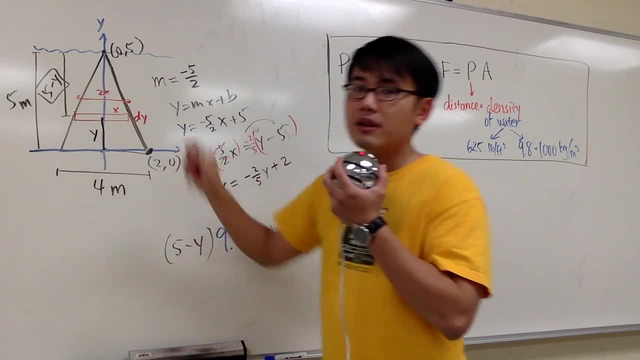 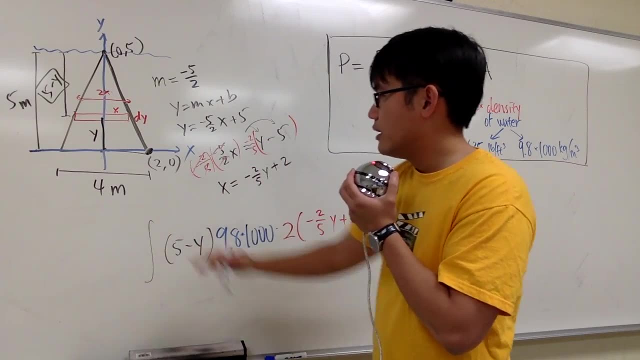 This right here will give you the force that's acting on this red rectangle here, and I just have to integrate the very first one till the very last one. So I'll integrate this. The very first one will be: y is equal to 0.. 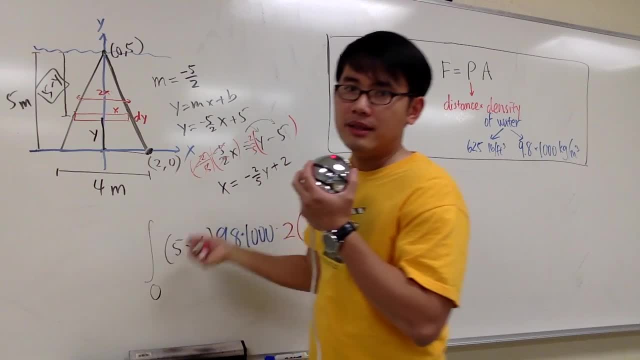 And the very last one, already on the top, is when y is equal to 5.. 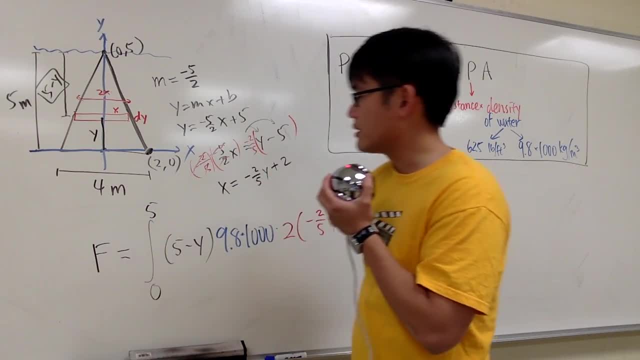 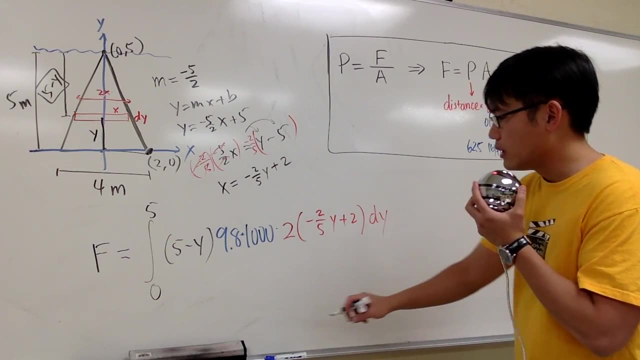 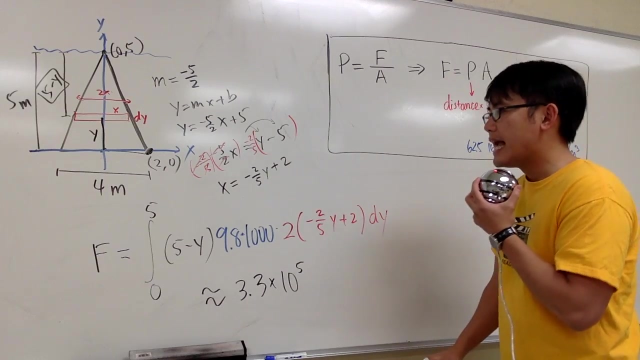 So that will be the integral And then that will give us the force for that triangular plate And we are done And the answer. once you worked out this integral, this is approximately 3.3 times 10 to the 5th power. 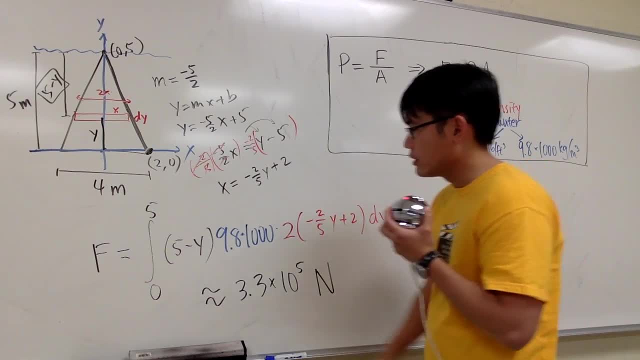 And we are using SI unit. The force will be measured in Newton. So this right here is it.